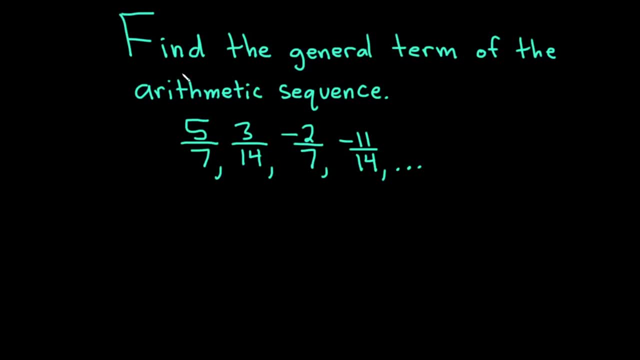 Hello, In this video we're going to do a problem involving arithmetic sequences. The question says: find the general term of the arithmetic sequence, And the sequence terms are 5 over 7, 3 over 14, negative 2 over 7, negative 11 over 14.. And the three dots indicate that it. 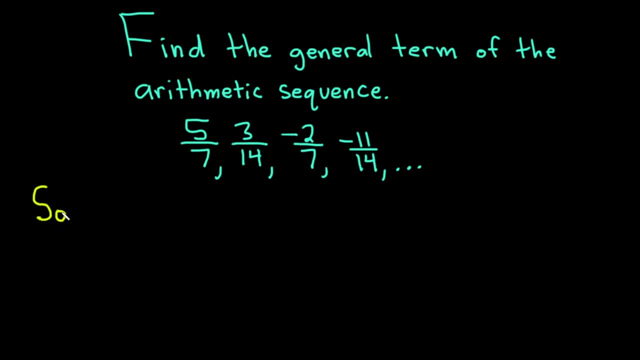 goes on forever. Let's go ahead and carefully work through this solution. Let's start by writing the sequence with a common denominator, So it looks like 14 is a good choice. We can take 5 over 7 and multiply it by 2 over 2.. The first term is really 10 over 14.. The second term is 3 over 14.. 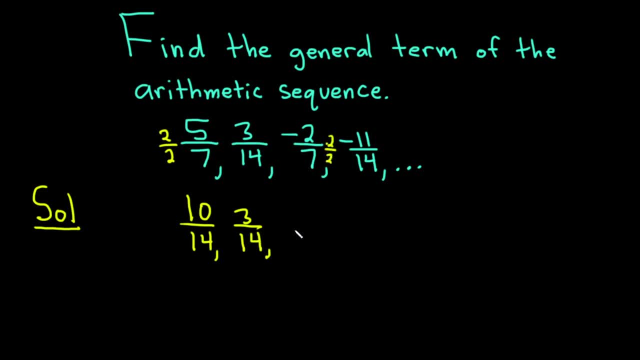 The third term. we can again multiply it by 2 over 2.. It would be negative 4 over 14.. The next one would be negative 11 over 14.. And then the three dots indicate that it goes on forever. So to find the general term, we need a few things. We need the first term. 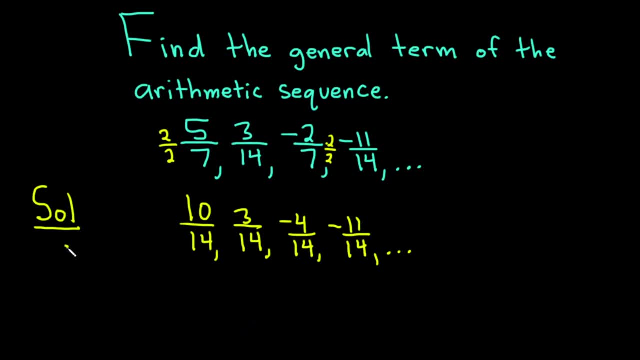 and we need the common difference. So a sub 1 is the first term, So in this case it's 10 over 14.. And the common difference is d. This is the number you add to get from one term to the next. 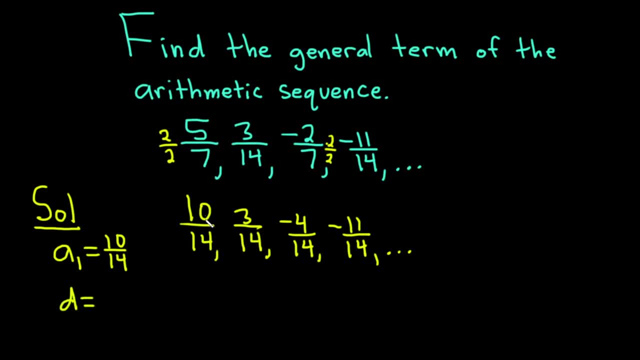 We can see here right away that, to get from the first term to the next, we're going to get from 10 over 14 to 3 over 14.. We're adding negative 7 over 14.. Likewise, to get from 3 over 14 to negative 4 over 14.. We're adding negative 7 over 14.. 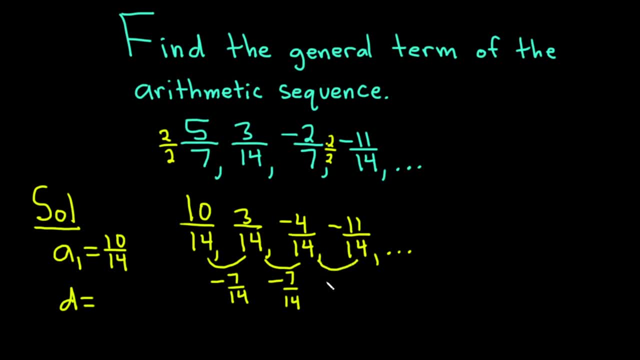 Same thing here: negative 4 over 14 to negative 11 over 14.. We're adding negative 7 over 14.. A little d is going to be negative 7 over 14.. So once you find your first term and your common difference, which is the number you add to get from one term to the next, 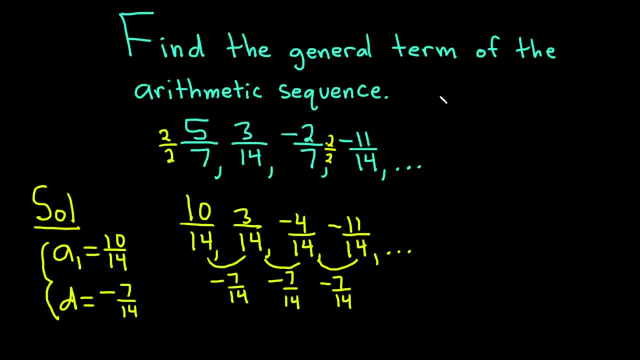 you can use your formula. so the formula for the general term of an arithmetic sequence, which is also called the nth term of the arithmetic sequence, is a sub n and it's equal to the first term, which is a sub 1 plus n minus 1 times d, so n minus 1 times d, or said another way, it's: 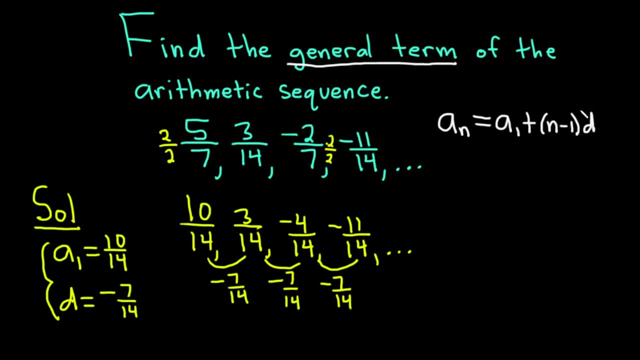 the first term plus n minus 1, common differences. d is called the common difference. so we have a sub: n is equal to so a sub 1, we said was 10 over 14. we replace a sub 1 with 10 over 14 and plus and we have n minus 1 and d is negative 7 over 14. so let's go ahead and replace that. 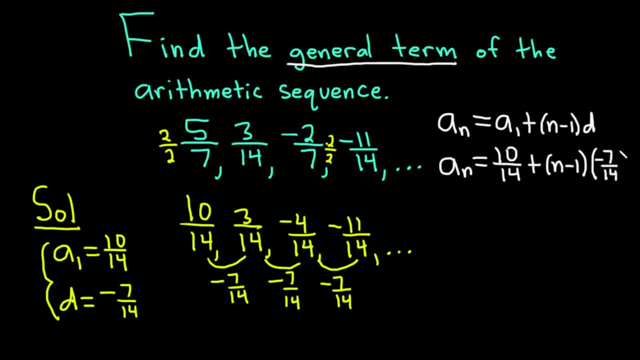 with negative 7 over 14 you. so a sub n is equal to. let's clean this up: this is 10 over 14. negative 7 over 14 times n is negative 7 over 14 times n and negative 7 over 14 times negative. 1 is positive 7 over 14. 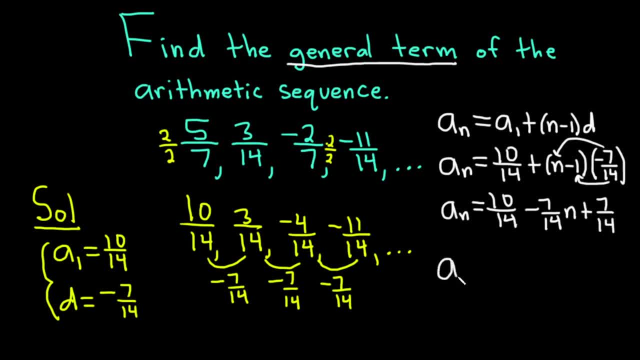 so finally we have a sub: n is equal to 10 over 14, plus 7 over 14 is 17 over 14. so finally we have a sub: n is equal to 10 over 14 times n is negative. 7 over 14 times n is negative 7. 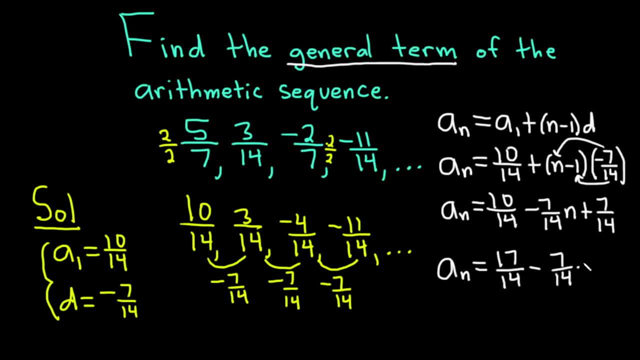 minus. and then we have seven over 14 times n. so the general term, or the nth term of this arithmetic sequence would be a sub n. so another way to know is to take the denominator, which is equal to, very similar to first. we've run these off. 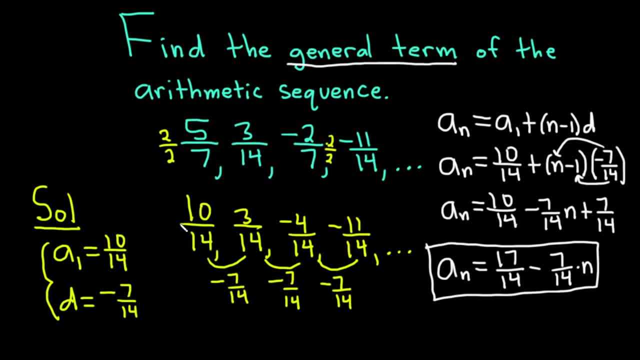 a sub n, we said the quantity is quiet. now we got our higher point where we wrote: n is equal to plus 7 over 14, minus 7 over 14 times n. so a bit messier than a lot of other problems, but hopefully we've kind of drew some planning hours into this work, so let's go ahead and multiply those. 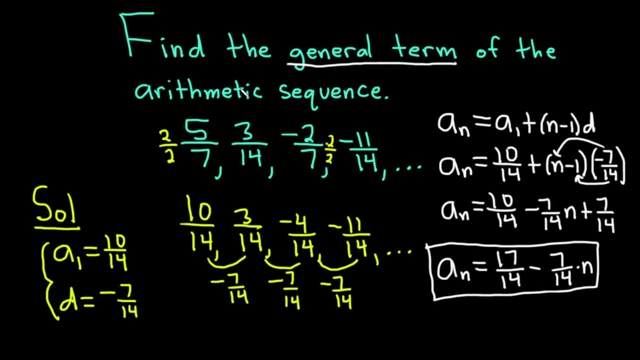 but hopefully it's been helpful next time. oh, i just realized something. this will be very much uh coupled with overhead equalization, so my first gente is going to be- i'm gonna talk calmly in- just about the second, i'm gonna use a calculator time. Oh, I just realized something Before we finish. we can do some simplification here. So 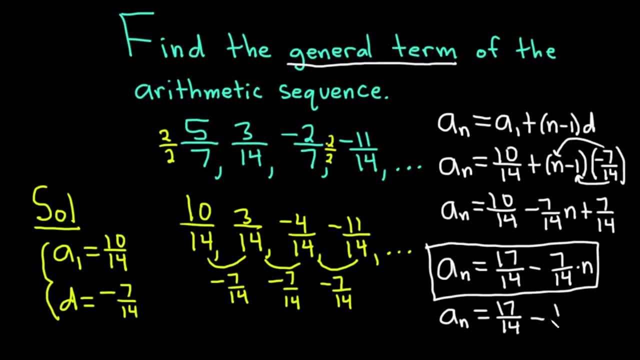 7 over 14 is really one half, So we can write it like that. So, yep, A lot of times you'll want to simplify your answers almost messed up there. So you can write 7 over 14 as 1 over 2 to clean it up. I hope this video has been helpful. Good luck.